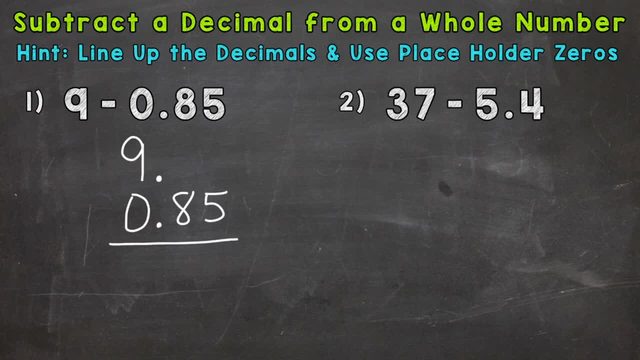 there lining up our decimals. We can put our equal sign and subtraction sign. So lining up the decimals there will line up all of the places for us. Now that may look a little offset, but we can use placeholder zeros so both of these numbers go to the hundredths place. Now I can place zeros to the right of a decimal because 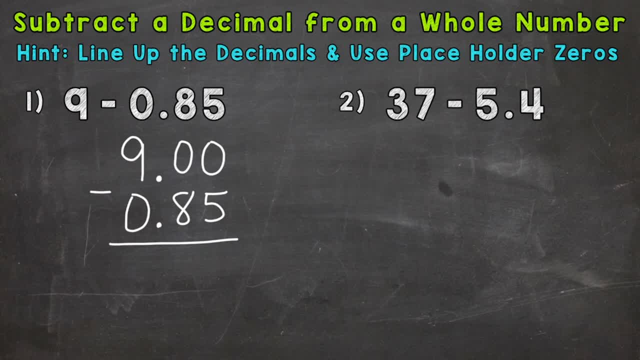 it doesn't change the value of that 9.. I didn't change the problem at all: That 9 still has a value of 9.. So now we just subtract. Now one of the most common mistakes would be just dropping that 5 and dropping that 8.. 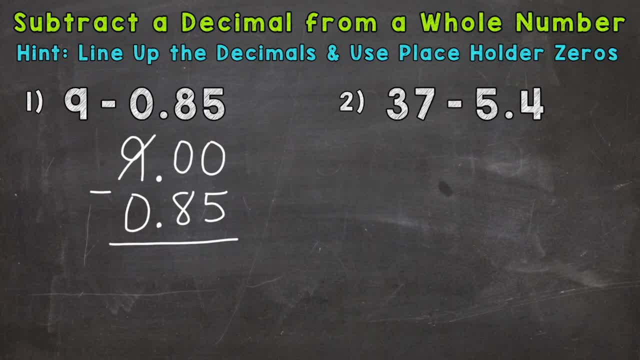 But we need to borrow. So we need to borrow from this 9. here That's an 8.. That becomes a 10, but we need to borrow again to bring that 1 over to the hundredths place. So now we have 10 minus 5, which. 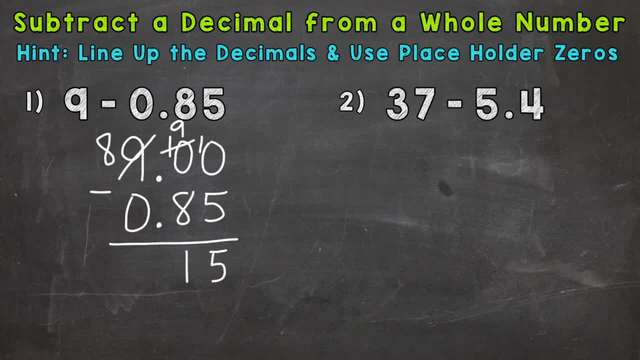 is 5.. 9 minus 8, which is 1.. Bring your decimal straight down so the decimal is lined up throughout the whole problem. Now, 8 minus 0 is 8.. And that's our final answer: 8 and 15 hundredths. 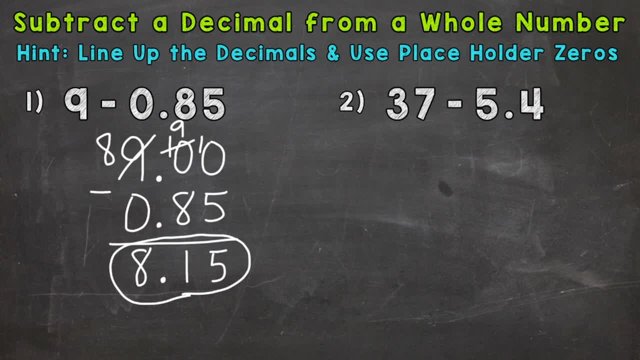 So let's go to another example here, number 2, where we have 37 minus 5 and 4 tenths. So the first thing we do line up the decimals And remember the decimal comes after any whole number. So now we can line up the 5 and 4 tenths And we can use a placeholder zero here, So both numbers. 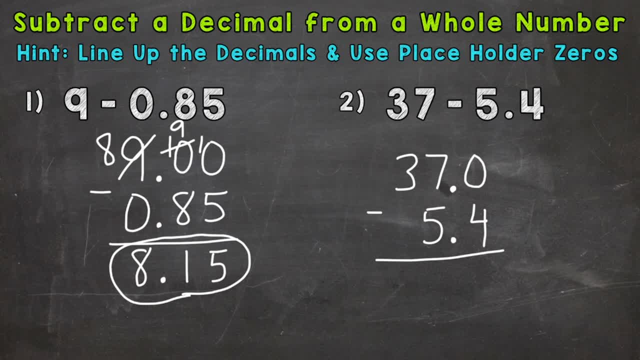 go to the tenths place And remember: the most common mistake is just dropping that 4 without borrowing. So we need to borrow from the 7.. So it's a 6 now And we end up with 10 minus 4, which is 6.. 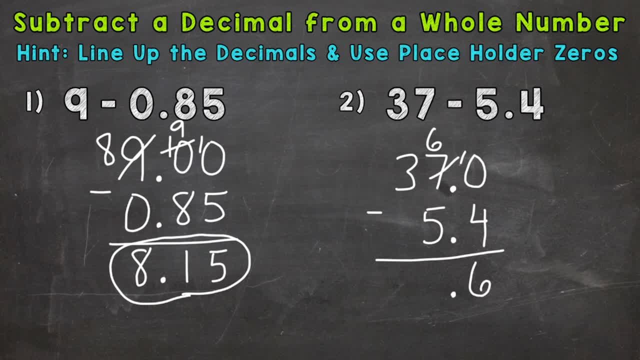 Bring your decimal straight down. It's lined up throughout the whole problem. 6 minus 5 is 1. And we have a 3 over here, So we end up with 31 and 6 tenths. So there you have it. There's how you. 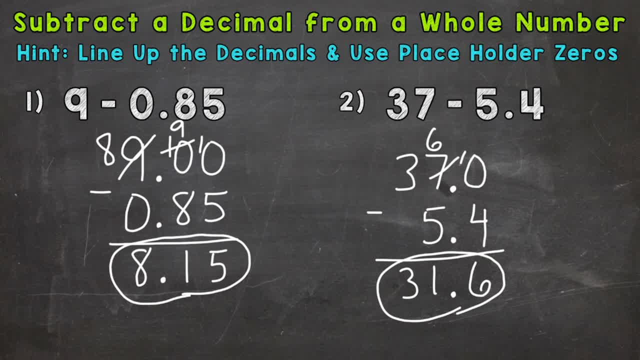 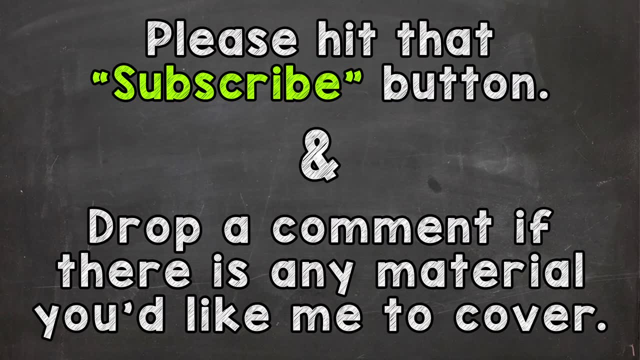 subtract a decimal from a whole number. Line up your decimals, Use placeholder zeros And subtract. I hope that helped. Thanks so much for watching. Until next time, Peace.